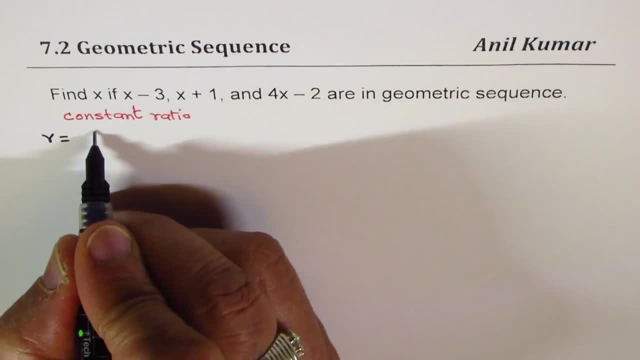 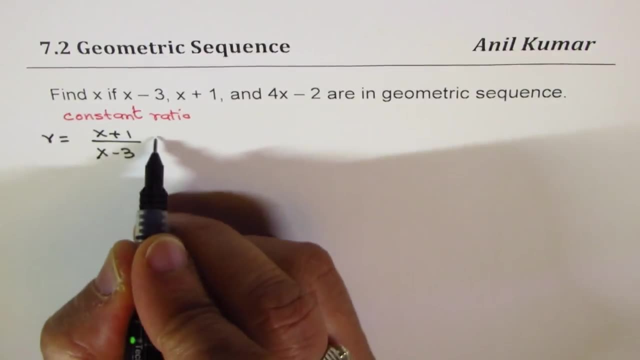 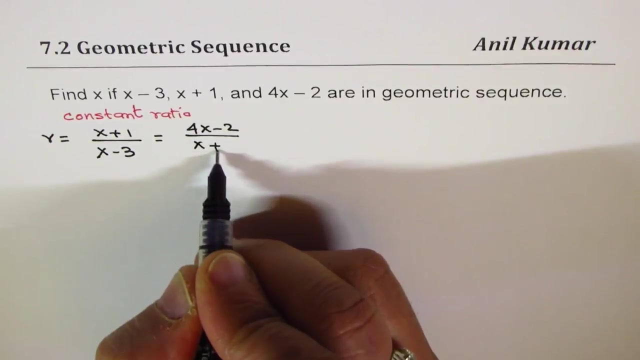 That is, if you are given three terms you could divide. You could divide x plus 1 by the previous term, which is x minus 3.. So that is ratio r. Similarly, you could divide 4x minus 2 by its previous term, which is x plus 1.. 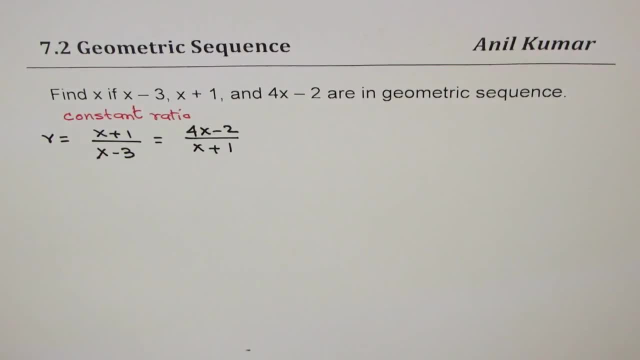 And all these ratios are equal. Let us say they are equal to r. So that is the very basic definition which helps you to solve this particular question. And now I think it is simple. You can pause the video answer and then check with my suggestions. 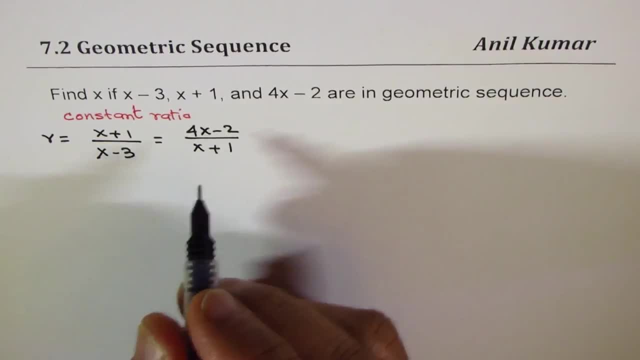 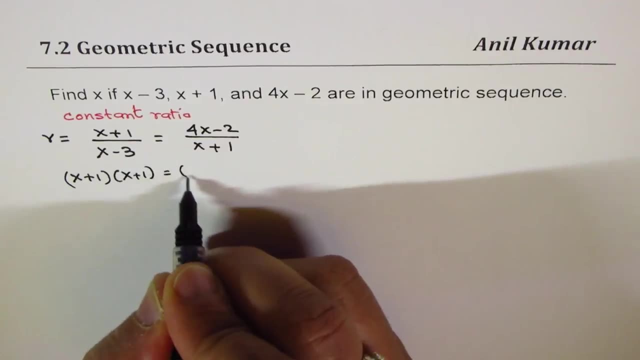 And now I think it is simple. You can pause the video answer and then check with my suggestions. We can cross, multiply, solve for x, We will get a quadratic equation. So we have x plus 1 times x plus 1 equals to 4x minus 2 times x minus 3.. 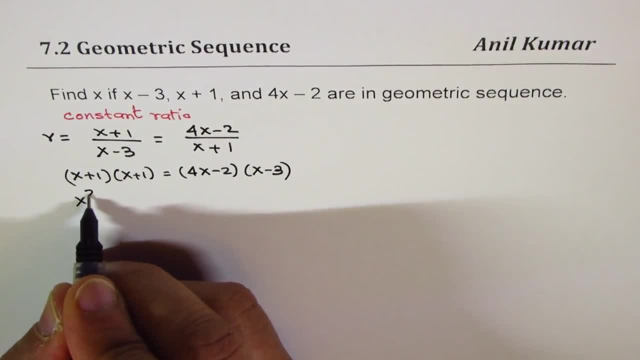 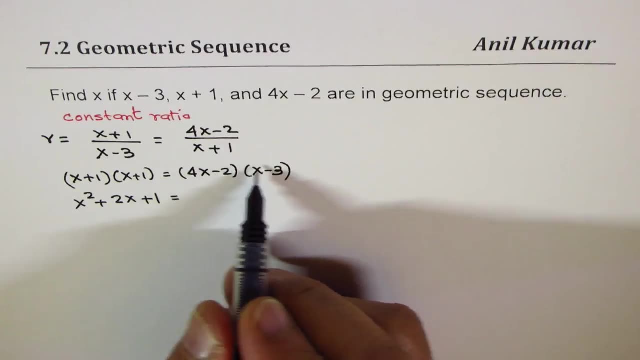 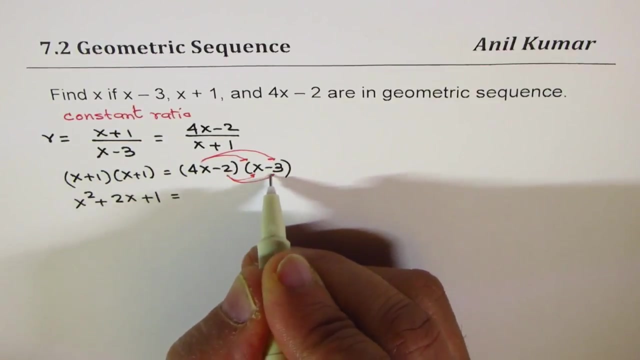 So here this is like square of x plus 1.. You could write this as x square plus 2x plus 1 equals to: let me multiply, this time Apply distributive property, that is to say Multiply both the terms with 4x first and then with minus 2.. 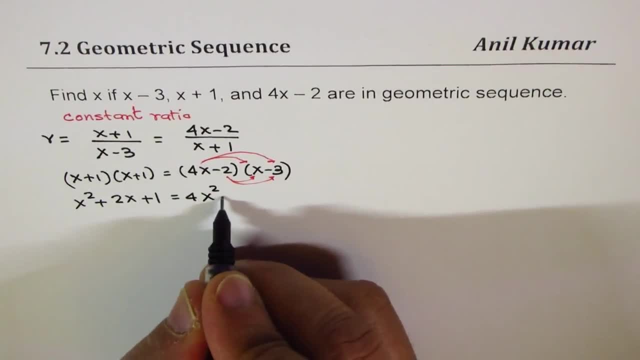 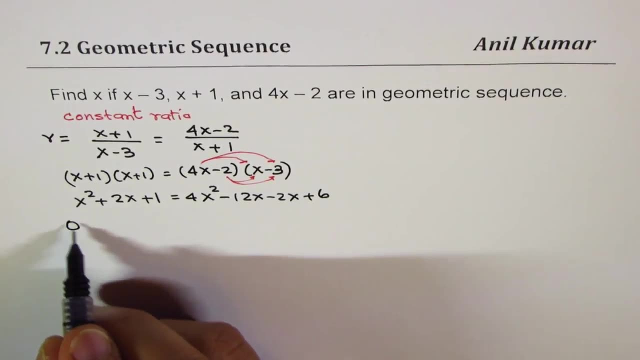 That will give me 4x square minus 12x minus 2x plus 6.. Now bring all the terms together So we could do 0 equals to 4x square minus 12 minus 2 can be combined, written as minus 4x plus 6.. 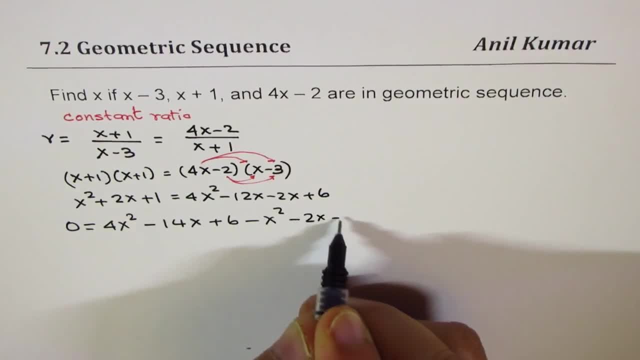 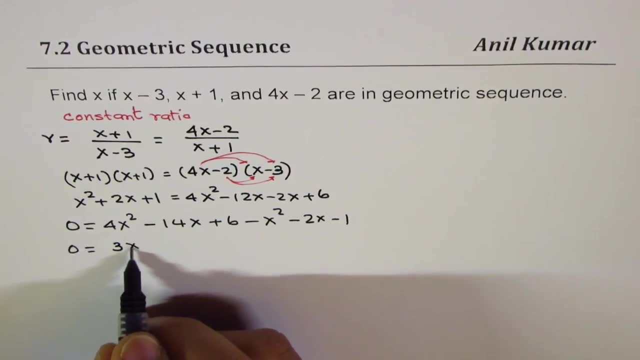 Take away x square, take away 2x and take away 1.. So that gives us 0 equals to 4x square. take away x square is 3x square. minus 14. minus 1 means minus. I mean minus 14 and minus 2 is minus 16x. plus 6 minus 1 is plus 5.. 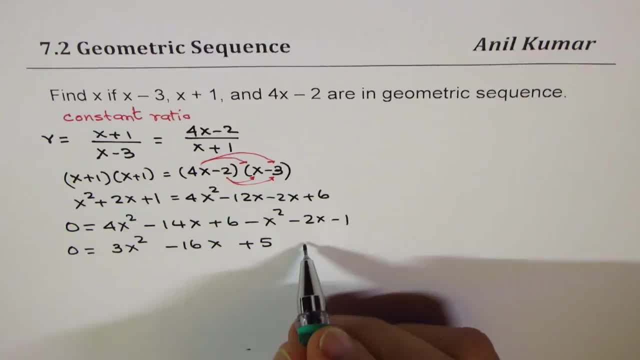 Now we are looking for product of two numbers. to factor whose product should be how much 5 times 3, which is 15.. And there Sum should be equal to minus 16.. Well, the two numbers are both negative, since product is positive, minus 15 and minus 1..